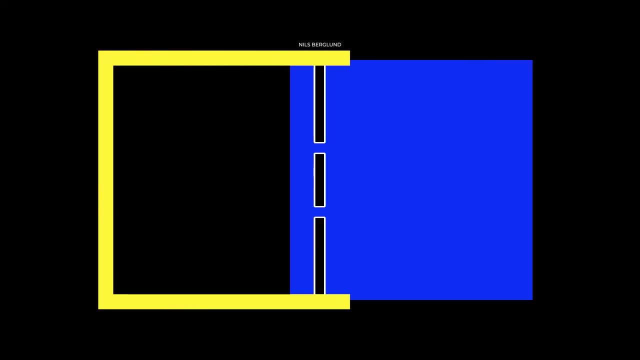 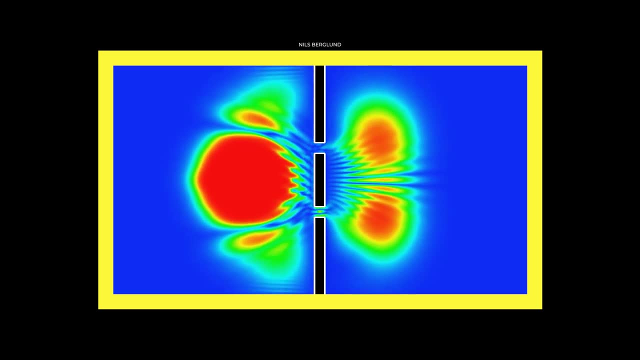 whether light behaved as a particle or a wave. When Young did the experiment, he showed that light that passed through two slits resulted in an interference pattern on the detector screen. Thus he found that light behaved like a wave and not like a particle as Newton had suggested. 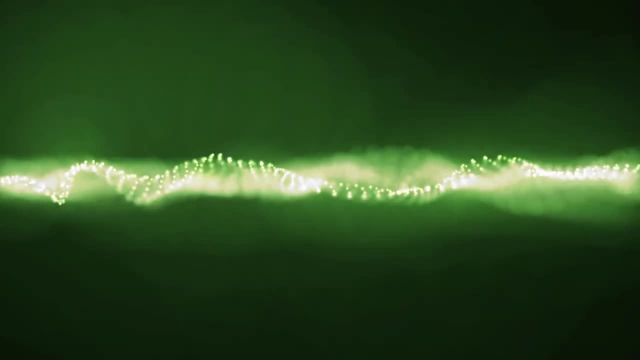 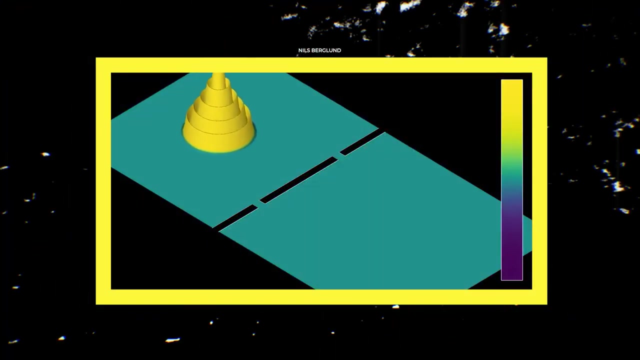 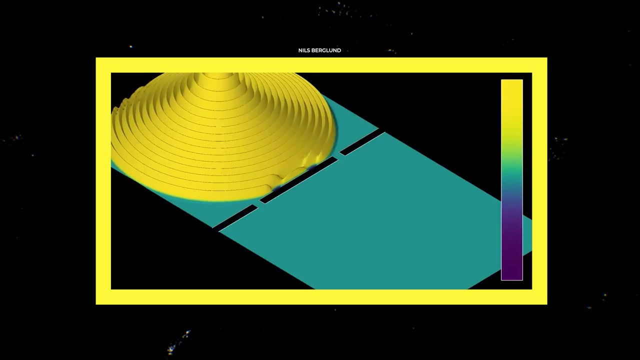 But not just light. any wave, whether it's a sound wave or waves across the water, can create an interference pattern. This experiment, however, is not that easy to make. If you want to see diffraction, the slit should be in the order of the wavelength of the light used. For visible light, that means 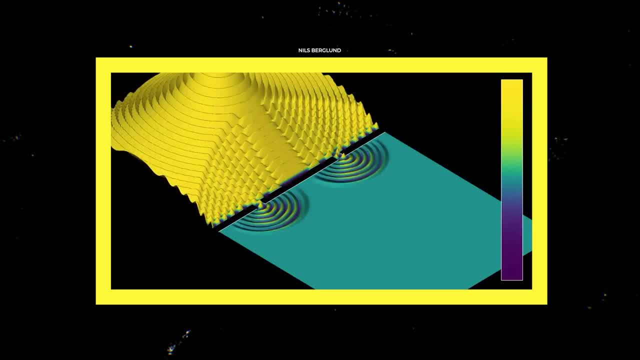 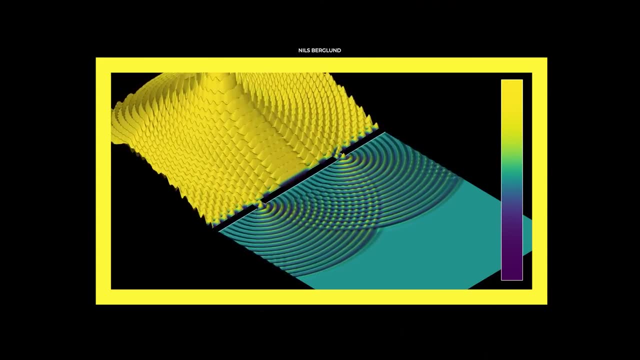 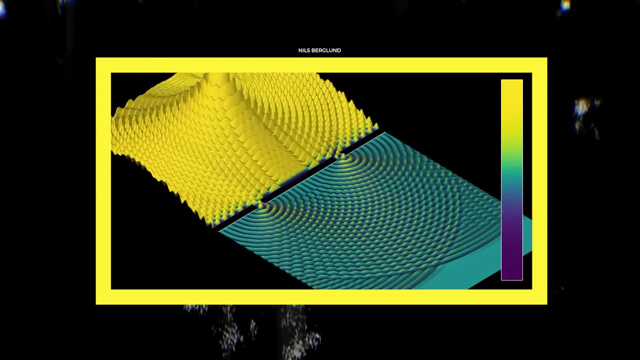 the slit should be on the order of less than one micrometer or one millionth of a meter. So light is a wave right? Not exactly. And here comes the mind-blowing part of this experiment. When particles such as photons or electrons go through the two slits, they create the same. 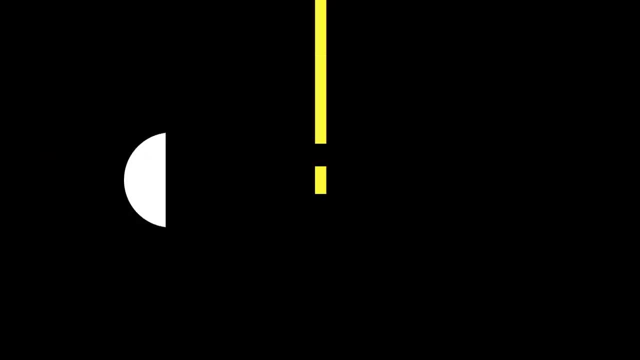 interference pattern on the back wall, as waves do, But when they're observed, they cast a two-slit pattern on the back wall. When they're observed, they cast a two-slit pattern on the back wall. Isn't that crazy? The electrons appear to act like waves when you're not observing them. 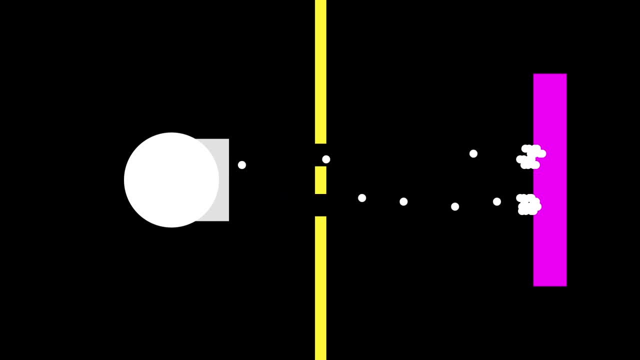 but as particles. when you are, It's like the electron knows that we are watching it. How, No one knows, And if you find out, please let me know in the comments. This shows that at a quantum level, light and matter can exhibit both particle-like 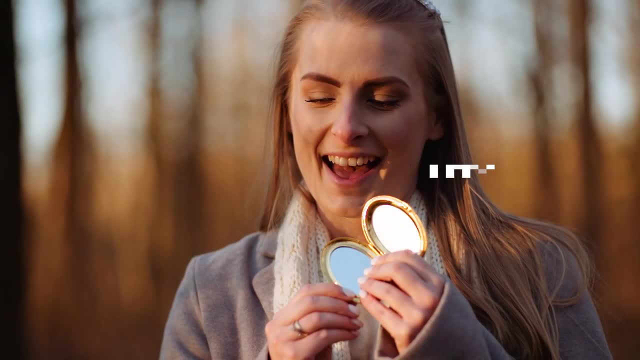 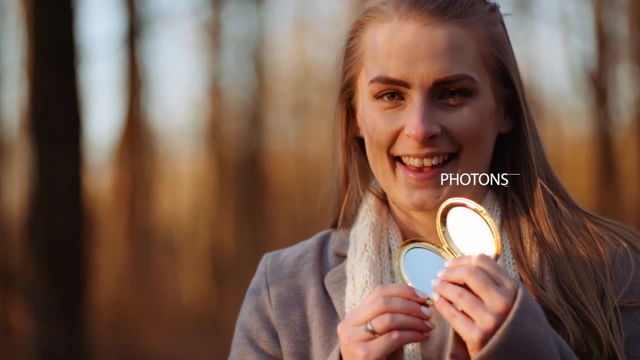 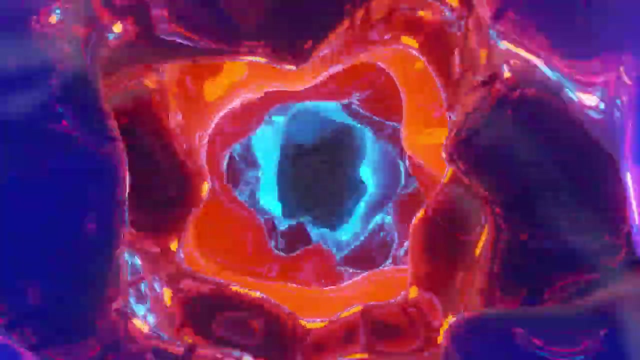 and wave-like properties. Light is made of quanta called photons. These quantum objects follow the rules of quantum mechanics, so they can behave as particles and waves. In the quantum field theory, objects are not particles but fields. Particles are unit excitations. of these fields, The lowest 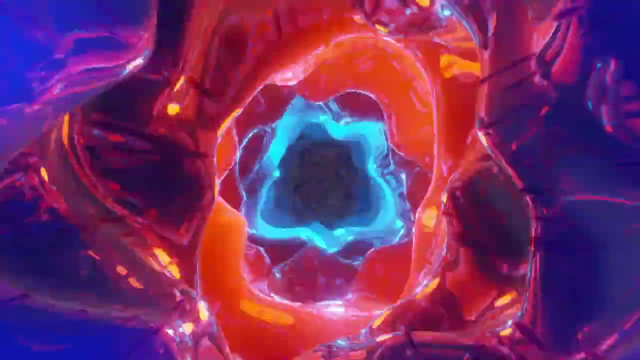 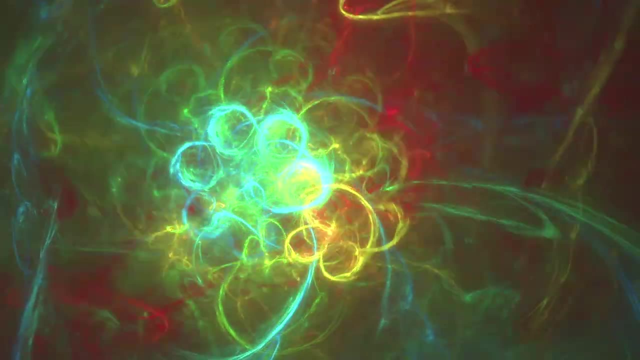 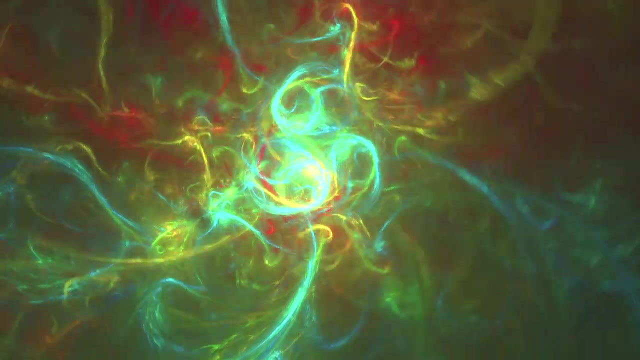 energy state of a field is when it has no excitations at all. This can't happen in the universe. we know For a photon to exist it takes a tremendous amount of energy. If there's no excitation in the field, there's no photon. Photons constantly vibrate and have momentum. 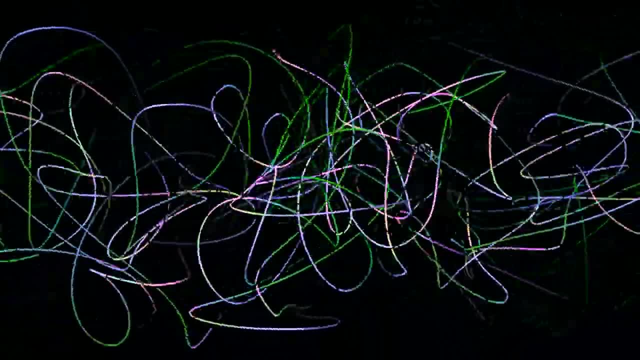 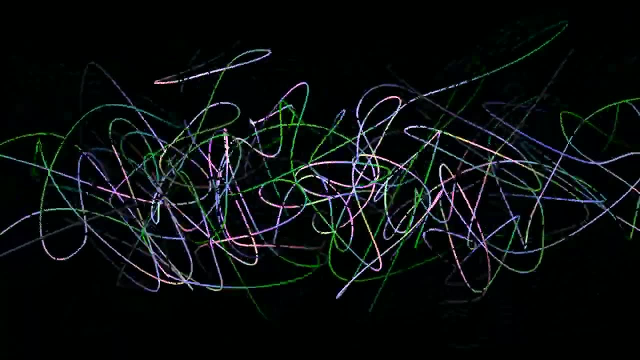 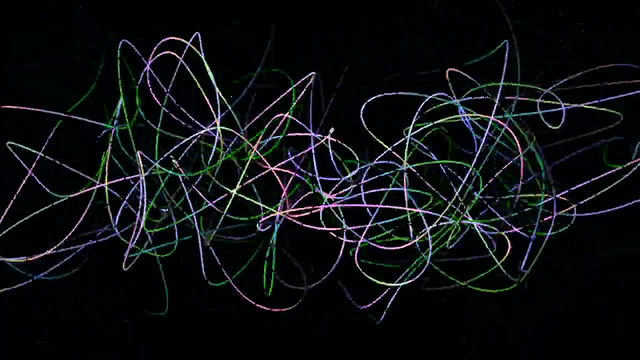 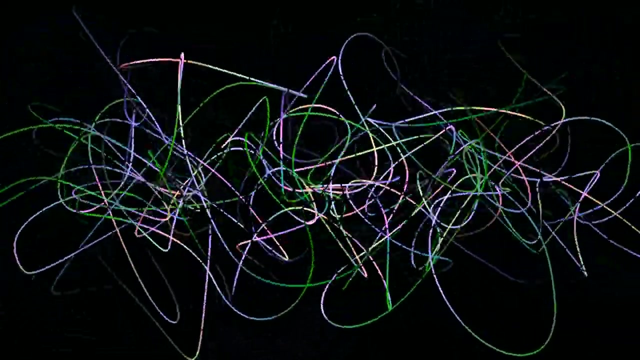 We are slowly starting to understand that particles don't even exist. There are no particles, only fields. And that's when string theory comes in. The string theory completely changes the standard description of the universe by replacing all matter-enforced particles with tiny vibrating strings that twist and turn in complicated ways. These strings are what?